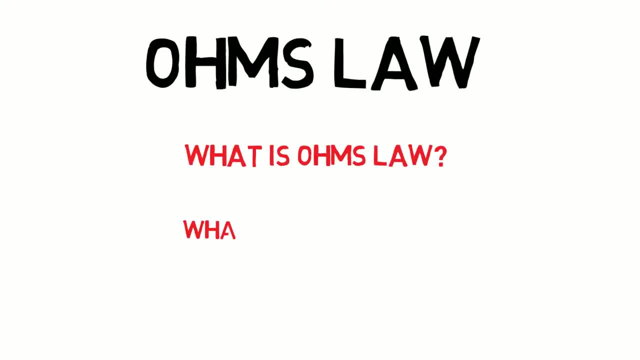 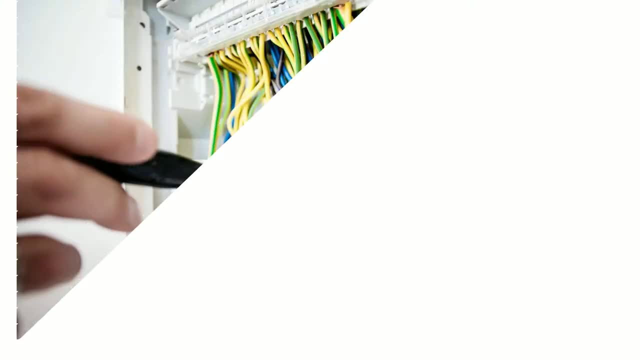 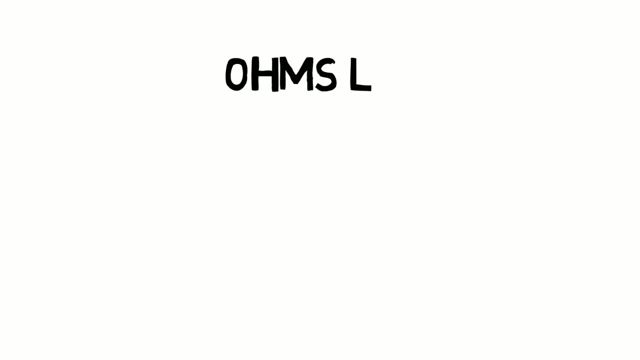 In this video we're going to discuss what Ohm's law is, show you what it is useful for and, of course, teach you exactly how to use it. Welcome back to Instrumentation Control. As an engineer or technician, you'll often be working on or designing electronic circuits. Ohm's law describes: 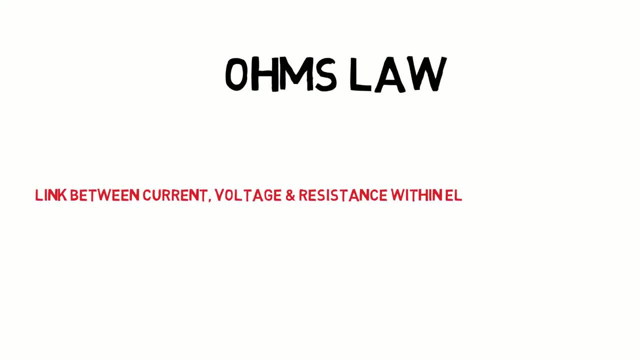 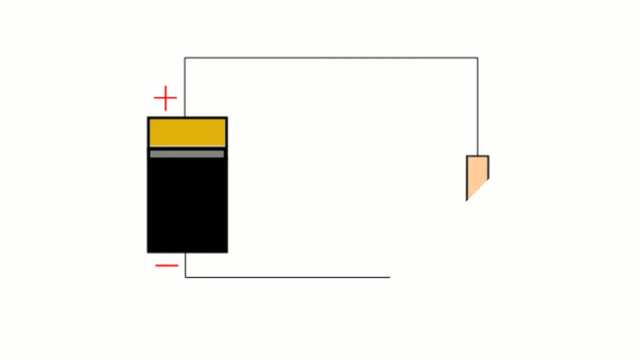 the link between current voltage and resistance within these circuits. If you aren't familiar with these concepts, there's a useful analogy that makes it all very clear. Let's take a look at the most basic electrical circuit of a battery, some connecting wire and a resistor: The battery. 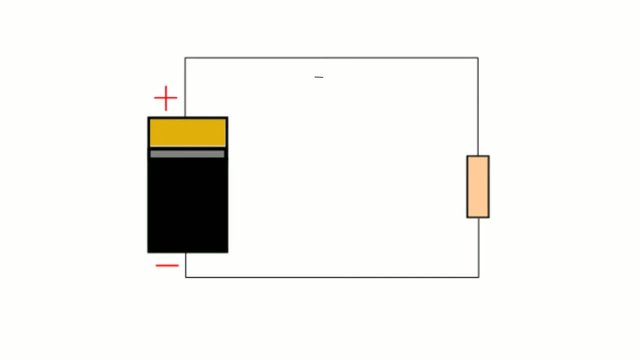 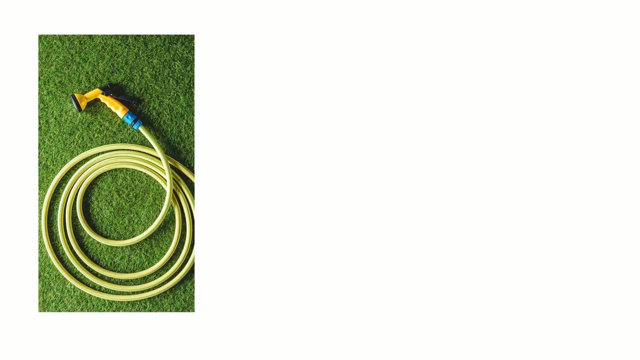 creates a potential difference of energy states or voltage that causes electrons to flow through the connected wire, the current that then travels through the resistor and back to the battery. The analogy that can help us understand this is your garden water hose. Think of a battery or voltage as the pressure. 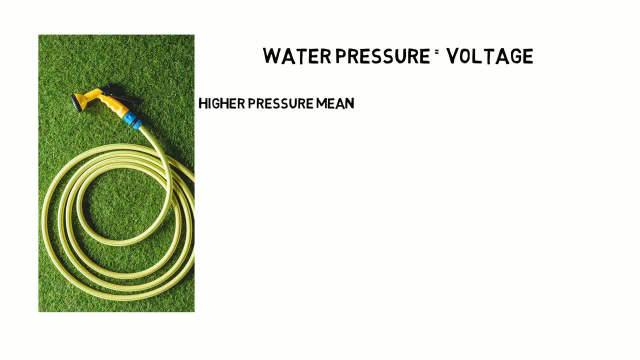 of your water supply. The higher the pressure, the more force is trying to push the water out of your outlet. The outlet valve is acting as a resistor by reducing the amount of water that can leave the outlet. The flow of water that does leave the outlet and through the hose can be thought of as: 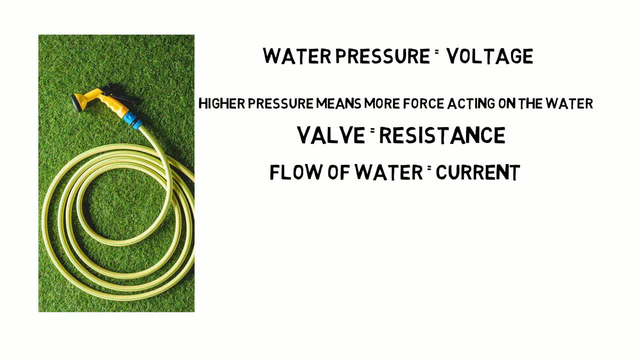 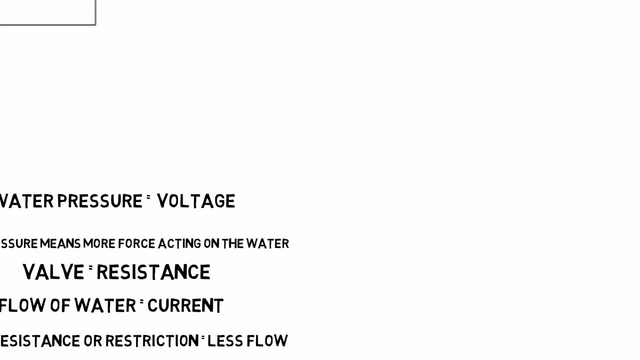 the current. All three of these properties are linked. If we increase the resistance or close the outlet valve off, then the flow is reduced. If we open the valve up or decrease the resistance, then the flow increases. Ohm's law describes the link between current resistance and voltage. If we know the 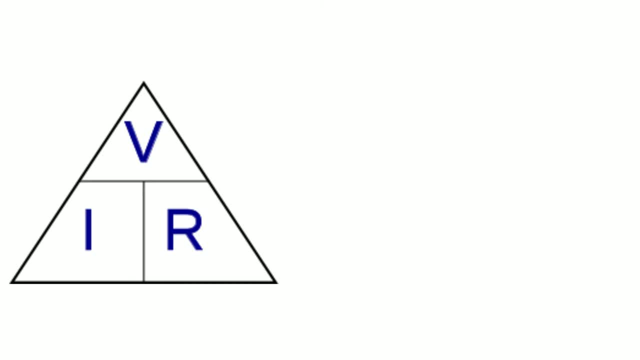 value of two of these properties, then we can calculate the third using Ohm's law. It's worth noting here that in engineering, voltage is denoted as V and measured in volts, Resistance is denoted by R or omega and measured in ohms, and current is denoted by I. 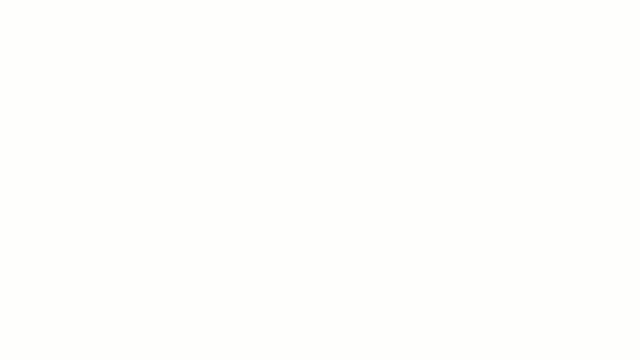 and is measured in amps. You'll often see Ohm's law written as a triangle like this. From this triangle we can quickly work out the formula for any of the three values by covering the value we're looking for and looking at the formula that we are left.